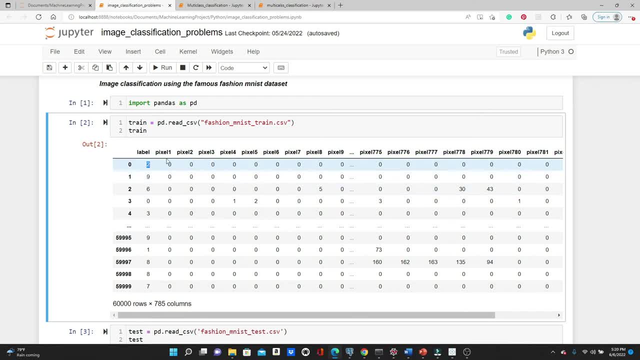 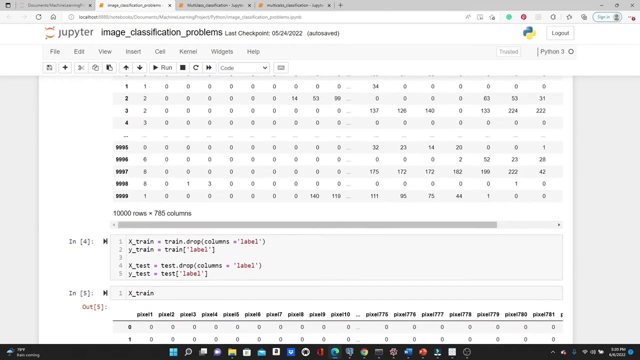 It could be a pullover, a t-shirt, anything. And then we have these pixel values in the same rows, from 1 to 7,, 84.. All these pixel values represent the pixels of the picture of that fashion item That's in label 2.. And here is our testing dataset. Here we are just separating the labels from the 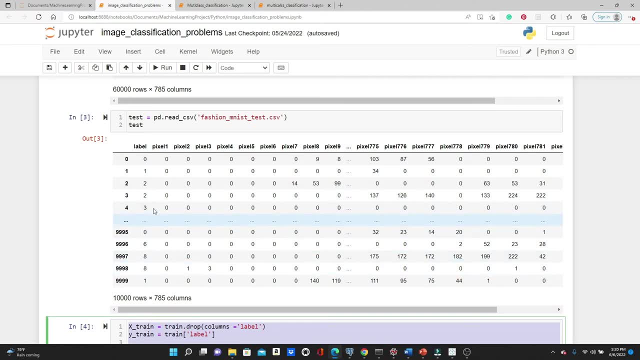 features Labels are literally this label column and features has to be these pixel values. The aim of this project is to make sure that the label column is the same as the features column. And the aim of this project is to make sure that the label column is the same as the features column. And 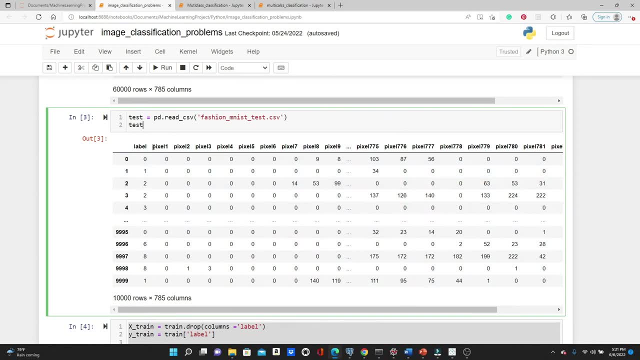 the aim of this project is to make sure that the label column is the same as the features column And was to train the model with these pixel values so that the model learns the pixel values and from the pixel values it knows which fashion item it was. 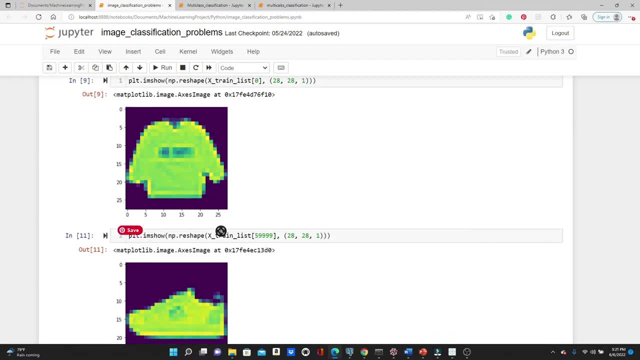 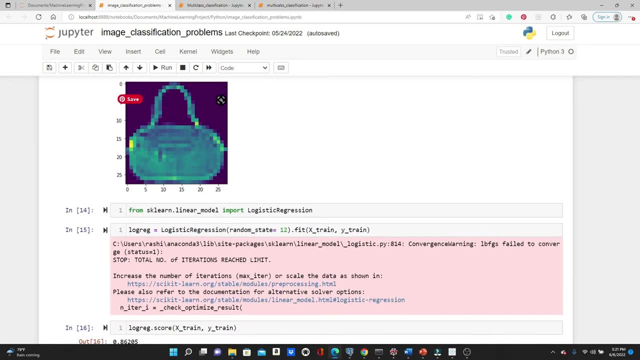 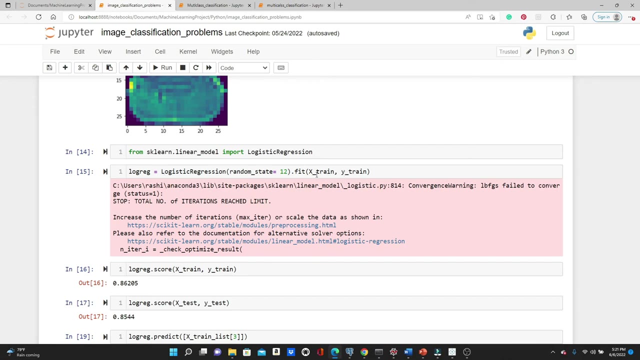 The next we wanted to see some of the pictures of these fashion items. This is a pullover and some shoes ankle boot. You can see this is a handbag. And then we imported the logistic regression from the psychic learn library. Then we trained the model using the training data. After that, 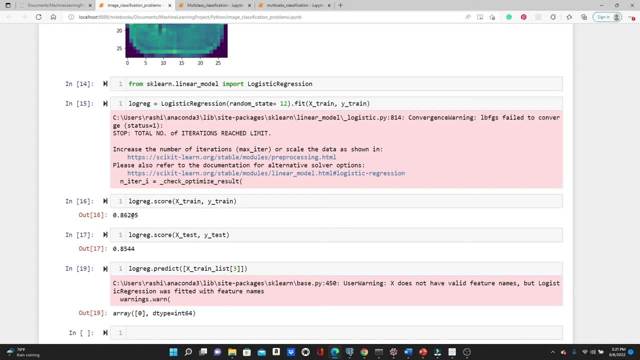 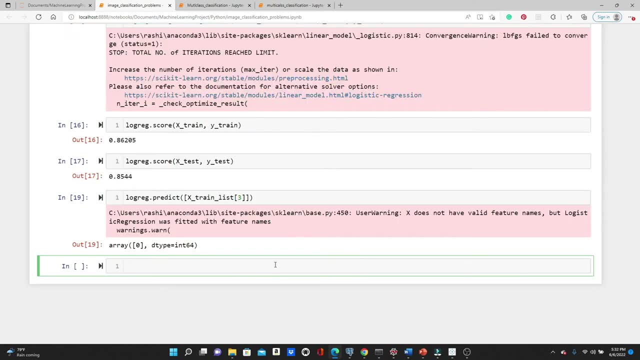 we got the scores. After that we got the scores For the training set, we had 86% accuracy and for testing data we had 85% accuracy. To get to the precision, recall and F1 score we need to find out. 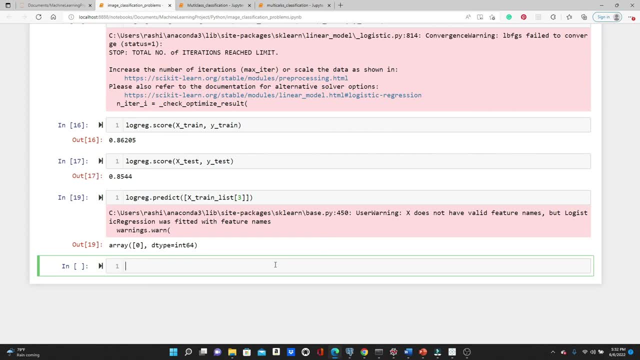 the Y prediction and also the confusion matrix. So let's see that Y print procedure. Red dot predict X test. Okay Now, the configuration is the same as the previous one, but it is different from the previous one, So we need to find out Y prediction and also the confusion matrix. Okay, Now the 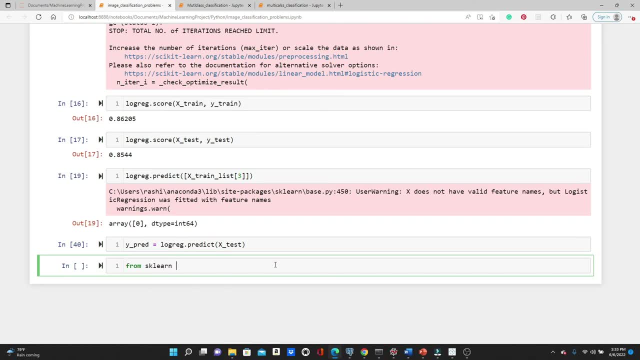 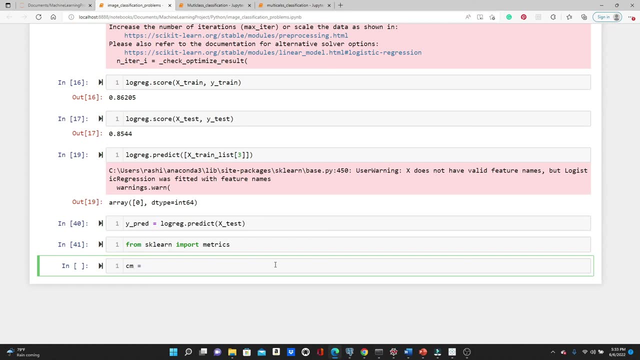 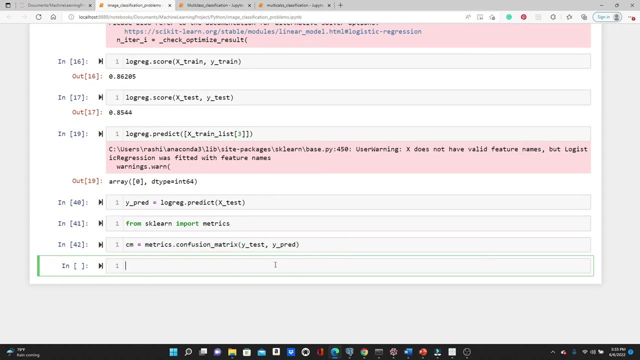 computation is the same as the previous one. So we need to find out Y prediction and also the confusion matrix. so first import escalern, import matrix. Okay, now the confusion matrix matrix, the confusion matrix, y test, the original y and y pred. Look at the. 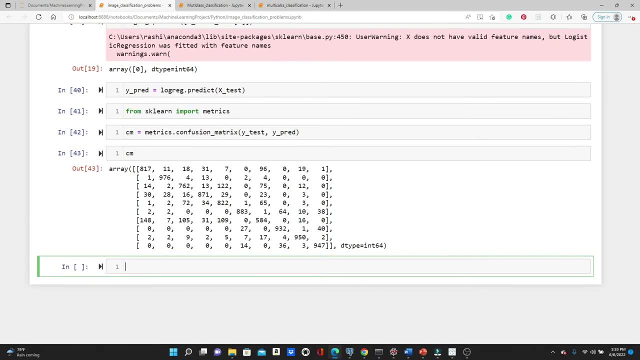 confusion matrix. Here is the confusion matrix. Look, when we did the binary classification, the confusion matrix was 2 by 2, because binary classification had only two classes, 0 and 1, and our, in this model, we had 10 classes. I want to. 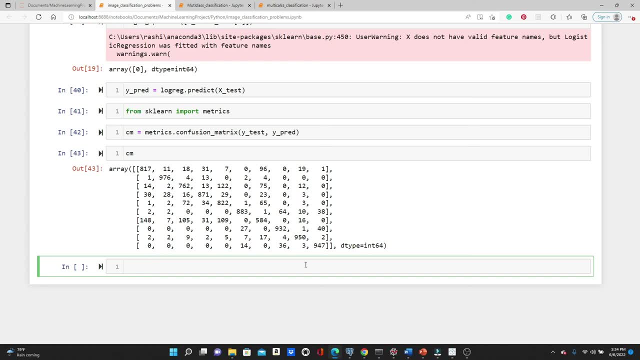 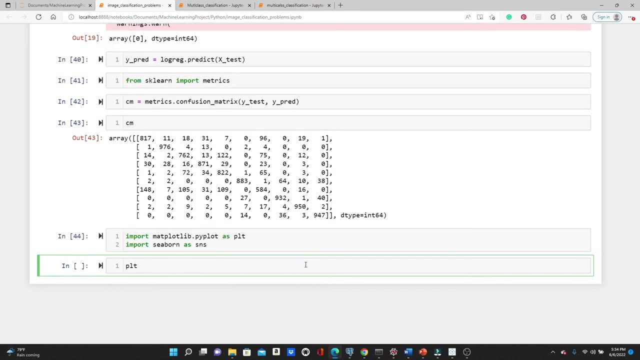 put this confusion matrix in a heat map so it will look nicer and more presentable. Import matplotlibpyplot as plt. import ceborn as sms. Plt dot. filev fixed size 9 by 9.. Now sms dot. the heat map, cm, not true. and now format 0.3f. 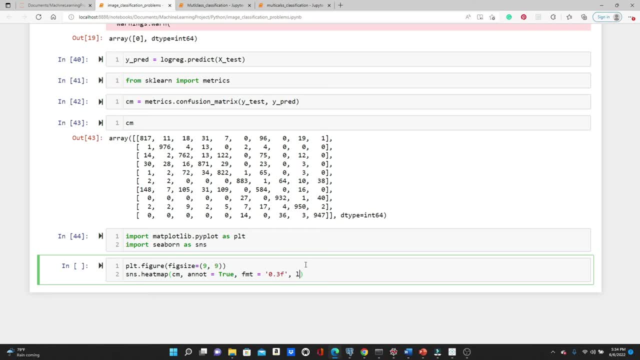 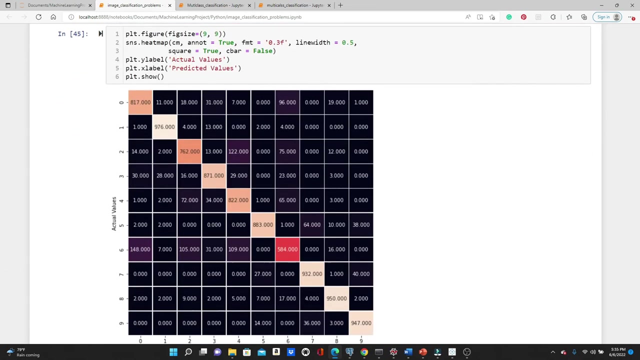 line width 0.5, square true, and we do not need any color bar and pltylabel. in y we have actual values and pltxlabel. these are the predicted values, pltshow. So here is the confusion matrix in a heat map. As you can see, it looks a lot more nicer and understandable. 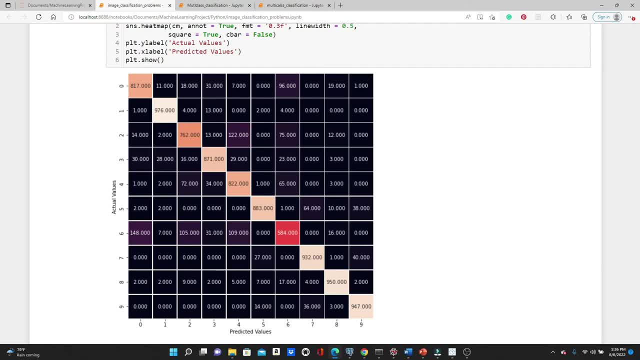 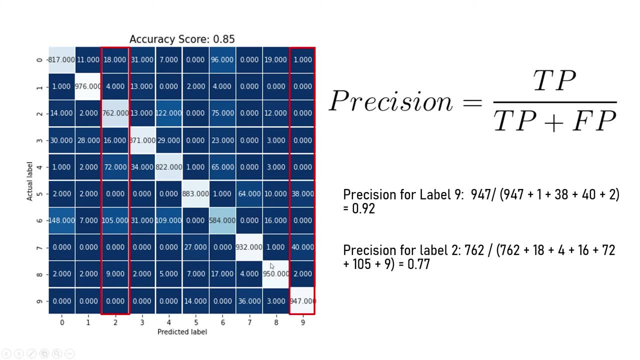 These are the predicted values in this side and actual values in this side. let's use this confusion matrix now. This is the same confusion matrix. I am just using a different color here. I hope you remember the formula for precision from my last video. 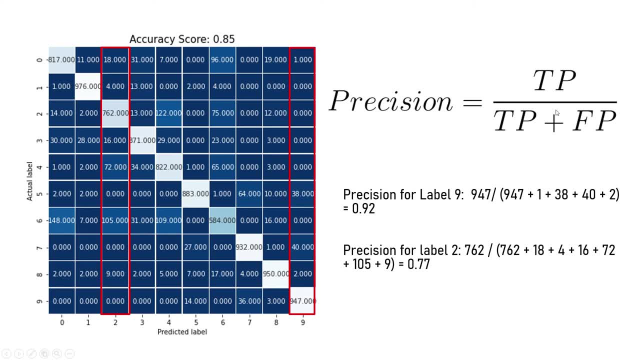 Precision is true positive over true positive plus false positive. So let's see how we can calculate precision for each label. Okay, let's take label 9.. What is true positive for label 9?? Look, this 947 was the predicted label for label 9. and again for label 9, we have this 947, true label or actual? 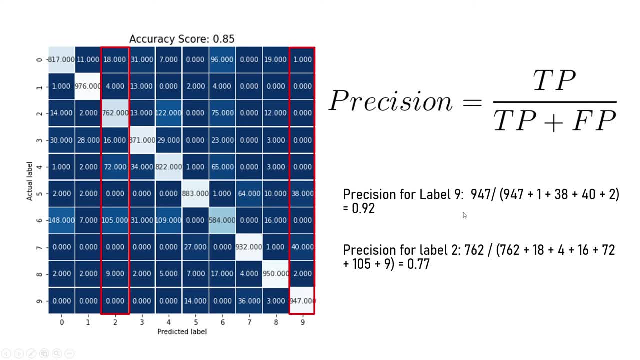 label. So 947 has to be the true positive for label 9.. So here we put 947 and bottom, also true positive, we put 947. here Now the false positive. What is false positive? Look at this. true, These two samples are actually label 8.. Again, these 40 samples are predicted as label 9, but they are. 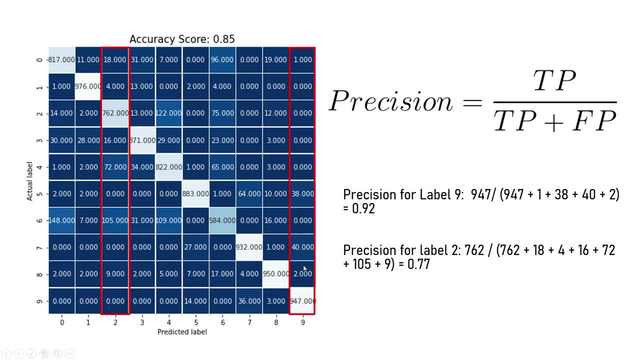 actually label 7.. So they are false positives for label 9.. So the false positive would be 1 plus 38 plus 40 plus 2.. Look, 1 plus 38 plus 40 plus 2, and so we have the precision of 0.92,, which. 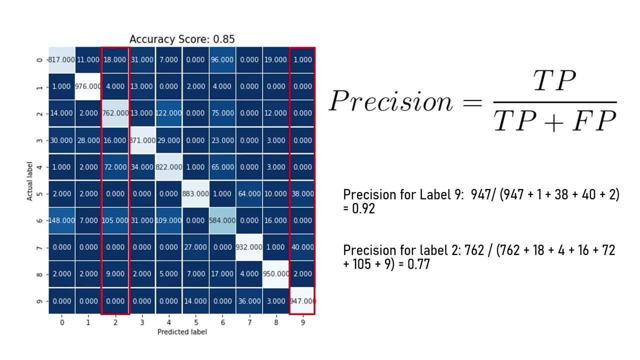 is really good. For the perfect case, precision is 1.. So in that case 0.92 is really high. Here we are calculating precision for label 2.. For label 2, true positive is 762.. Actual label 2,. 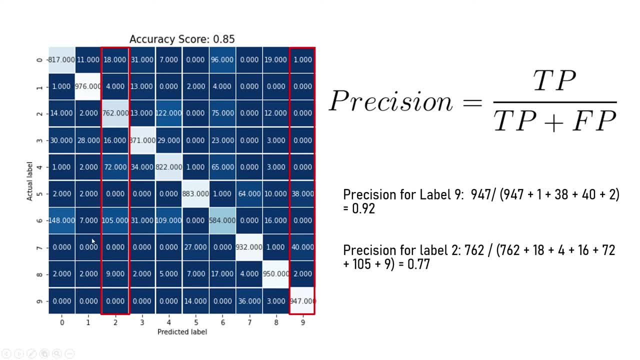 and we have 762 samples. Now, predicted label 2 is also 762 samples. So 762 are the true positives. So true positive over true positive plus false positive. let's see the false positives, these agent samples. this is actually zero, but our model predicted them. 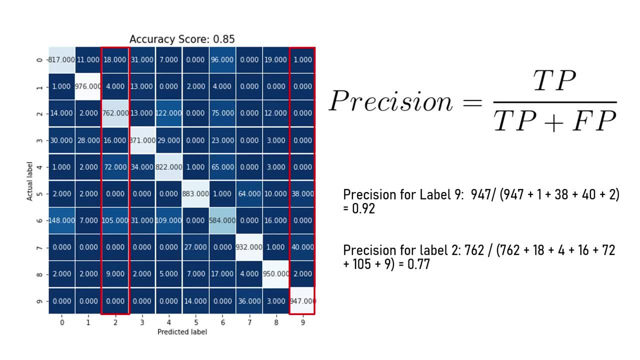 as two. so this agent samples has to be false positive for label two, four, this sixteen, seventy two, one, oh, five and nine. they all are actually predicted as level two, but actually they are not label two, they're label eight or six or four or one. so the false positives are 18 plus 4 plus 16. 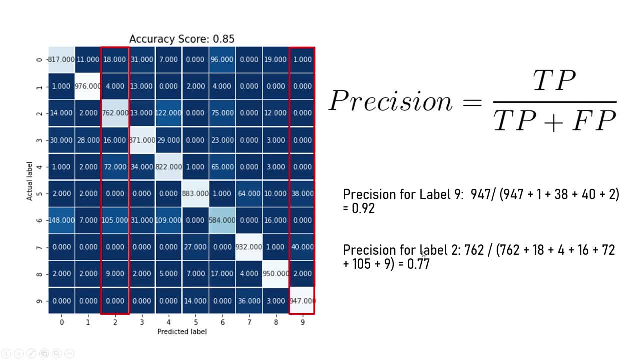 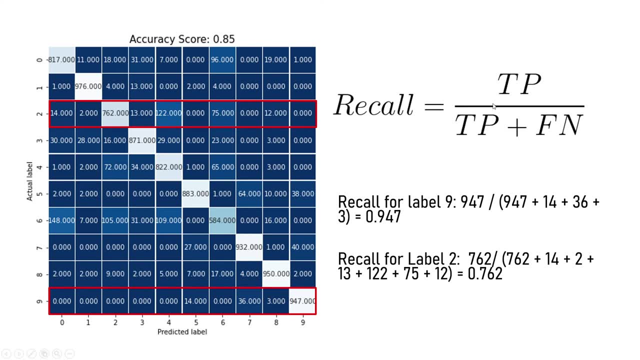 72 plus 105 plus 9 and it's 0.77. now recall: the formula for recall was true positive over true positive plus false negatives. so you also calculated recall for label 9 and label 2. as we already have seen, 947 was the true positive for label 9 and look at the false negatives this time. 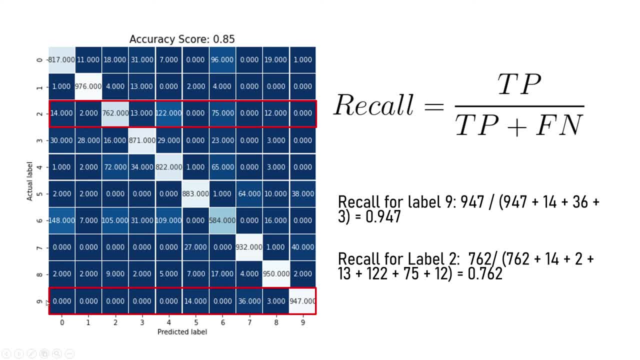 look at these three samples. it's actually label 9, but our model predicted as label 8. it didn't predict as label 9, so it was predicted as a negative for label 9. right, look at this 36. it's actually label 9, but our model did not predict them as label 9. 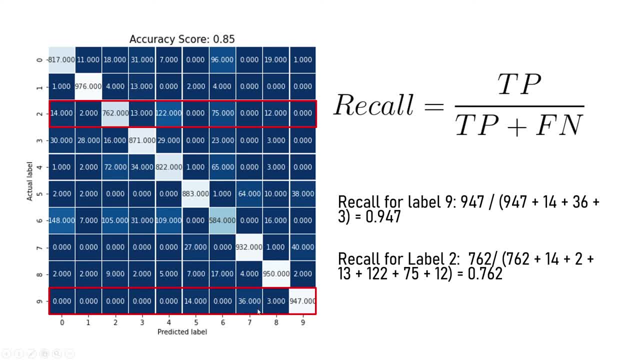 but our model predicted them as label 9. so for label 9 this 36 actually false negative. so the false negative has to be 3 plus 36 plus 14.. so recall is 0.947. so recall is very high. recall for label 2- as usual, you already know this- true positive was 762. 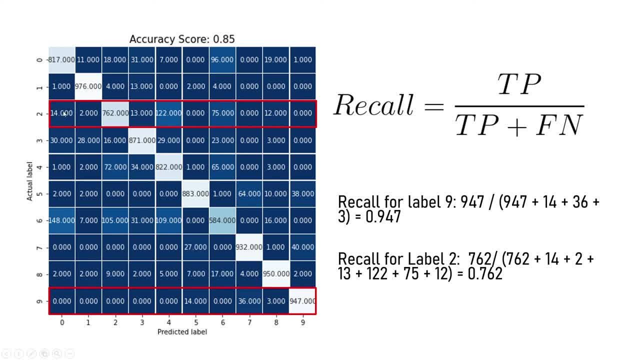 and then let's see the false negatives. look at this 14 samples. it's actually label 2, but our model predicted is level 0. So it did not predict it as level 2.. So for label 2, these 14 samples were. 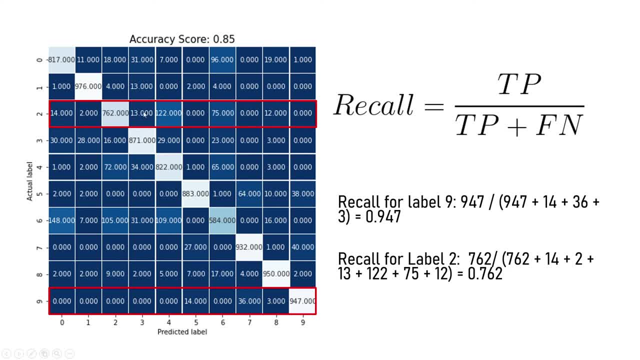 false negatives: Same as this 2,. same as this 13,, same as this 122.. So the false negatives has to be 14 plus 2 plus 13 plus 122 plus 75 plus 12.. The recall came out to be 0.762 for label 2.. 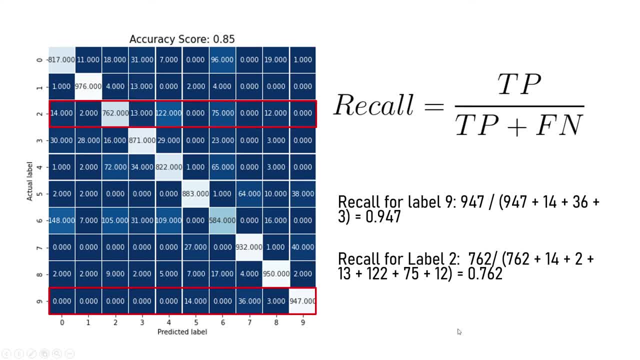 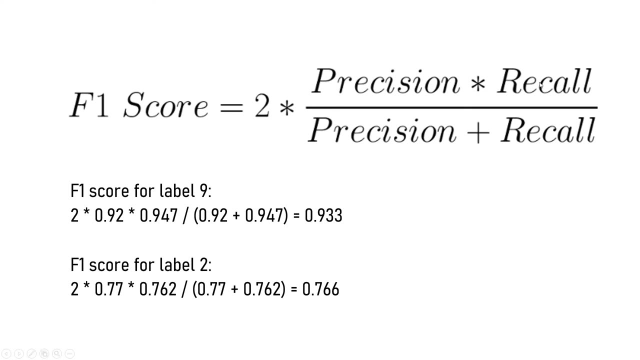 I am only showing precision and recall for label 9 and label 2 only, but you can use the same method and calculate precision and recall for each and every label, The F1 score. we are just going to calculate the F1 score using the simple formula: 2 times precision, times recall over precision plus. 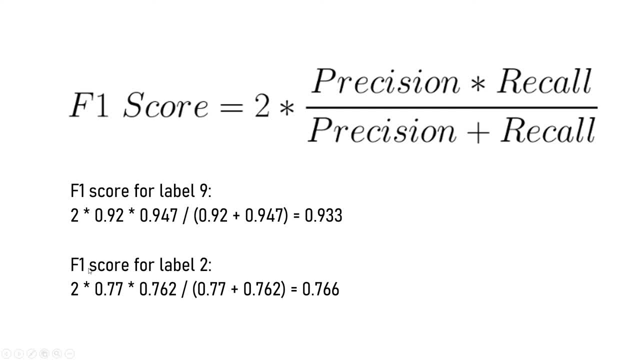 recall. So you can see for label 9, we have 0.93 and for label 2, we have 0.766.. As a reminder, F1 score is the harmonic mean of precision and recall And F1 score tend to lean towards the lower value between. 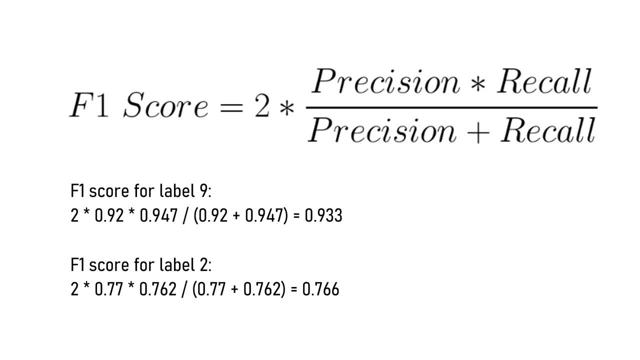 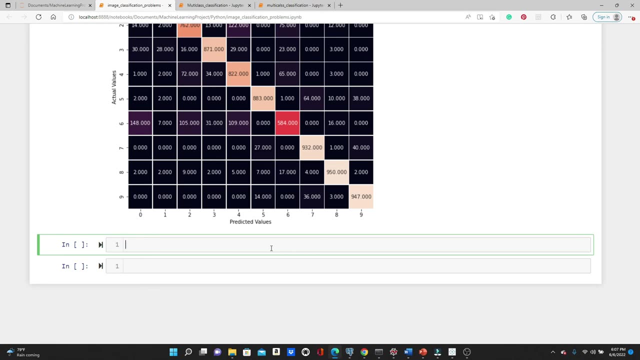 precision and recall. If either precision or recall one of them is 0, F1 score becomes 0. So to get a high F1 score, precision and recall both has to be high. The good news is you don't have to calculate the precision, recall and F1 score. that way You can use the simple line of. 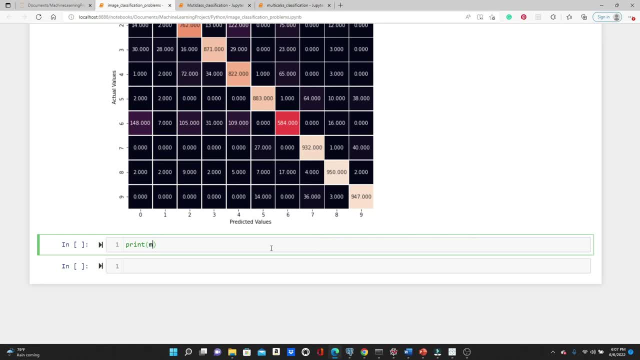 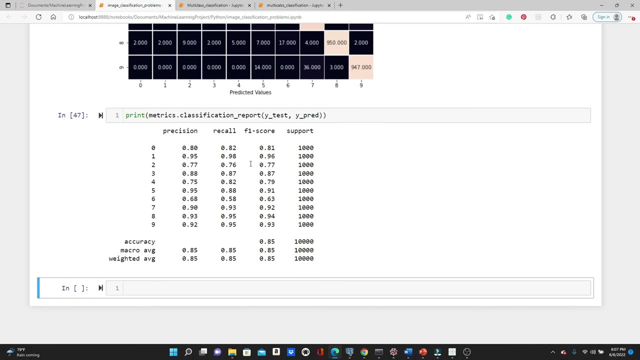 code. Print Now matrixclassification report. You simply give y test and y prediction And you can see the precision recall and F1 score for each label. We have label from 0 to 9. So we got precision. 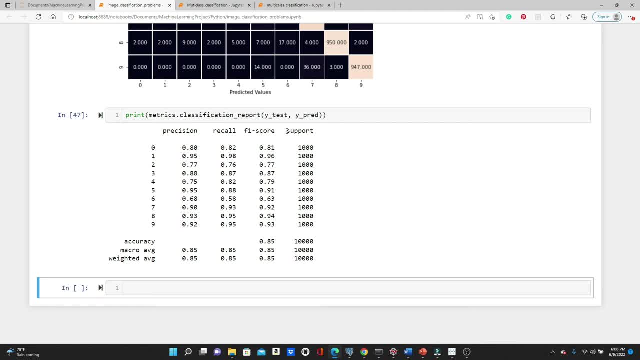 recall and F1 score for each label And you can see this support. These are the number of data for each label. We have 1000 data each for each label, So total, we have 10,000 data. Look, this is good to have. 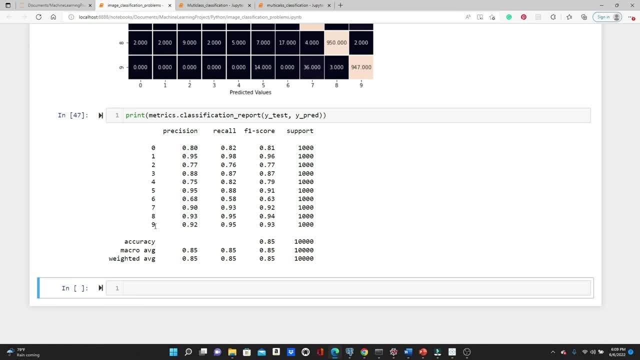 precision recall and F1 score for each label. But at the end of the day we still want one single precision recall and F1 score for a certain model. So for the overall model we have the precision of 0.85.. 0.85 was the recall and F1 score also 0.85.. So for the overall model we have the. 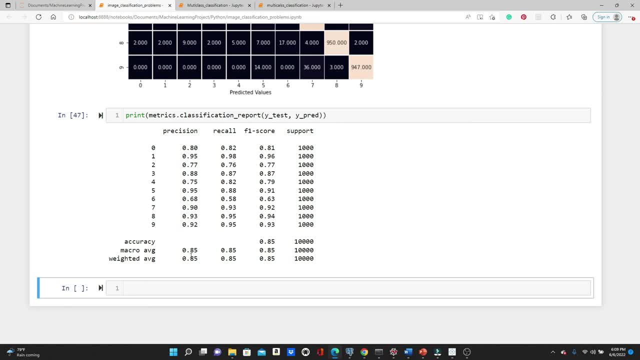 precision recall and F1 score also 0.85. Luckily. And weighted average also 0.85,, 0.85 and 0.85.. Now look how to calculate this macro average and weighted average: precision recall and F1 score. 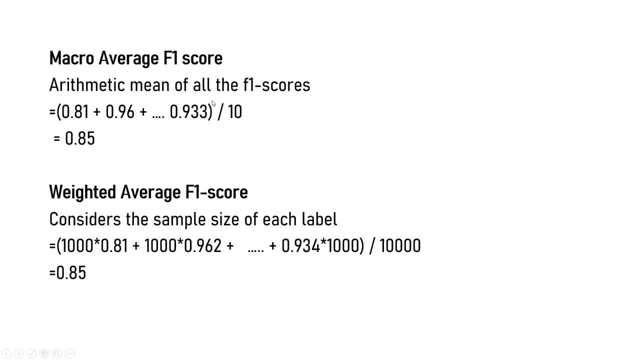 The macro average F1 score is actually the arithmetic mean of all the F1 score. We have 10 F1 score for 10 labels. So simply you add all the 10 values and divide it by 10.. That's how we get macro. 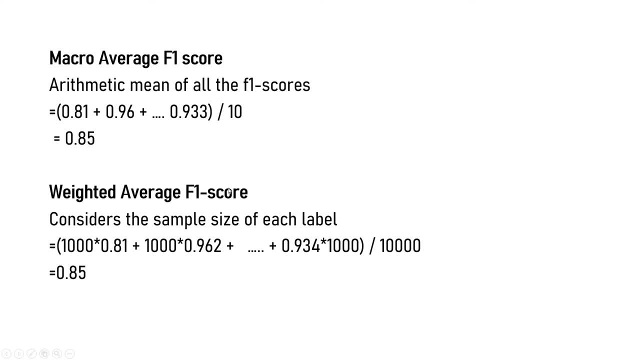 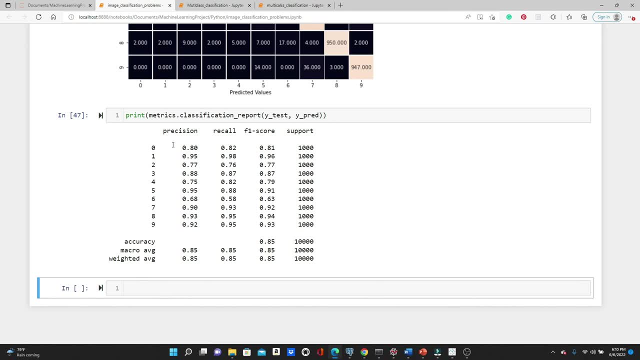 average F1 score 0.85.. And the weighted average F1 score takes into consideration the number of samples. We have the same amount of data for each label. For 0, we have 1000 data. For 1, we have. 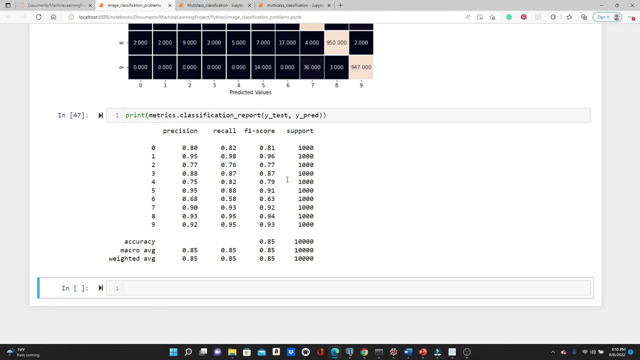 1000 data And for 9, we have 1000 data- all 1000, right And over we have 10,000 data. So luckily, we have 1000 data each. That's why macro average and weighted average are exactly the same, But it 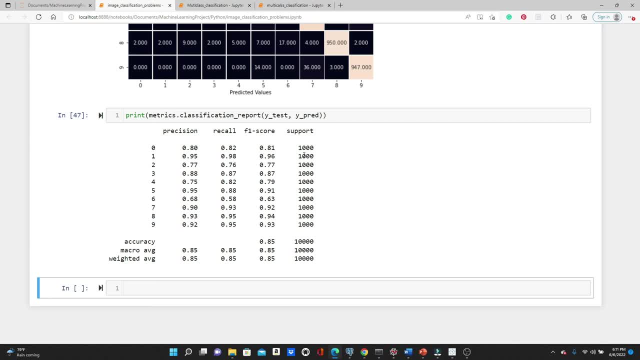 doesn't happen in most of the cases. In most real world data set, we have different number of data for different labels. In that case, macro average and weighted average F1 score can be different. Look at this weighted average F1 score.